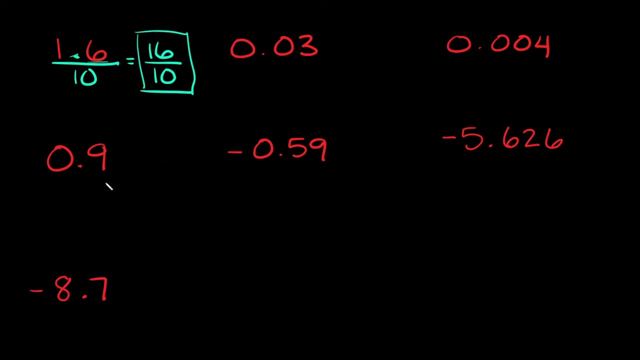 try another one. So here we have 0.9.. So again, all you have to do is figure out which decimal place value does this end in. Well, this ends in the tenths place, right? So I'm going to draw a line under my whole number and it ends in the tenths place, So I'm just going to write a 10 in. 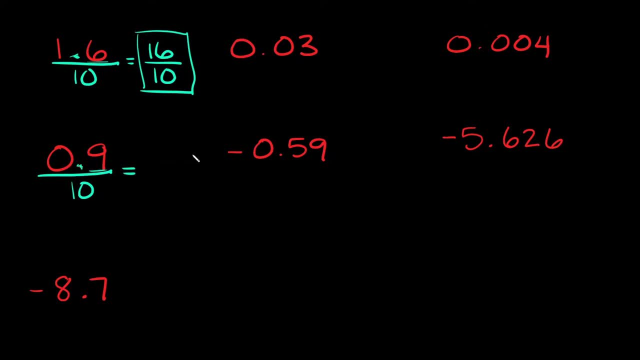 the denominator. Okay, so here's my fraction, right? So if I wanted to write it out here again, I'm just going to drop the decimal. So I'm just going to have 9 over 10.. So 0.9 as a fraction would be 9. 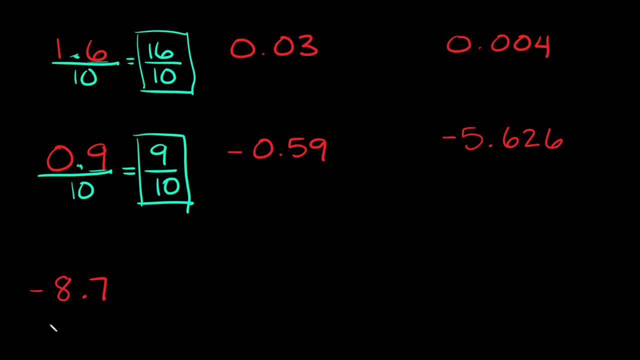 over 10.. Okay, now this next example. you can see it has a negative number, right, But nothing changes. All right, it's still the same process: gonna check to see what is the last decimal place. Okay, so it ends right here in the tenths place, so I'm just gonna put this whole thing over a 10.. Okay so. 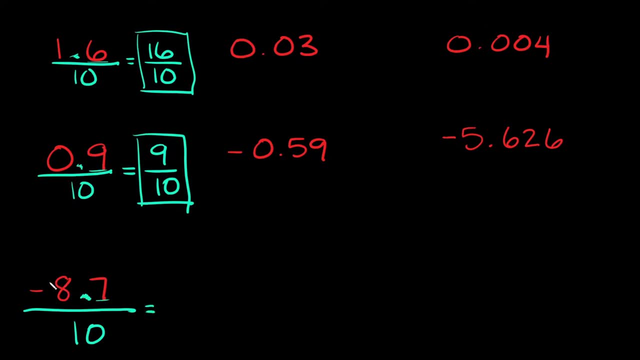 my answer would be: remember, just drop the decimal up here and then write your whole number. so we're gonna have negative 87 over 10.. Okay, so this would be your answer, right there. Okay, let's go to the next example. so here we have 0.03. 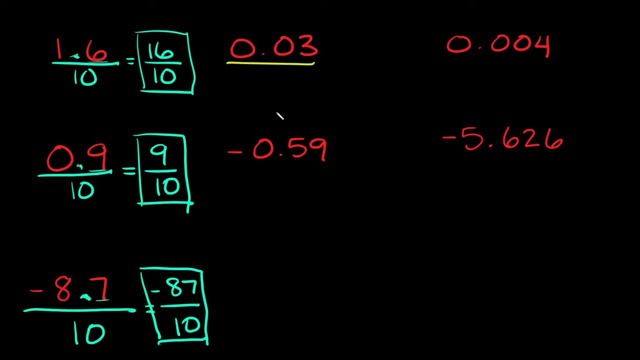 so just draw a line underneath the whole thing and then what place value does it end in? Well, let's see, this is the tenths, this is the hundredths, so it ends in the hundredths. so I'm gonna put a hundred in my denominator. Okay, so I'm. 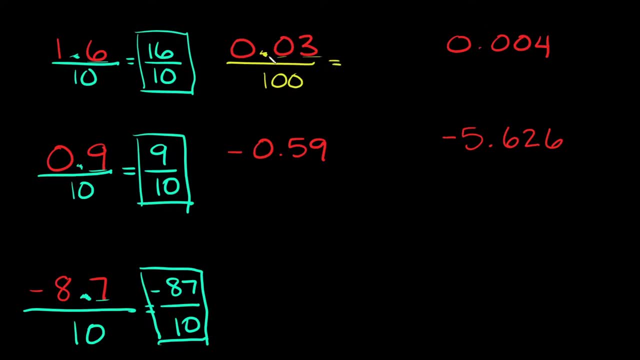 gonna rewrite my answer and again all I have to do is drop the decimal. so up here I'm gonna have 0, 0, 3, or in other words just 3, right, and then in the denominator 100.. Okay, so 0.03 as a fraction would simply be 3 over 100. Okay, next example: again, we have a 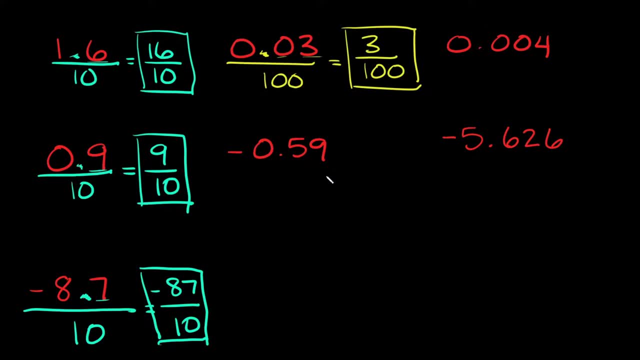 negative number right here, right. so negative 0.59.. So all I'm gonna do is draw a line underneath my whole number and then what place value does it end in? Well, let's see, this is the tenths, this is the hundredths and that's where it. 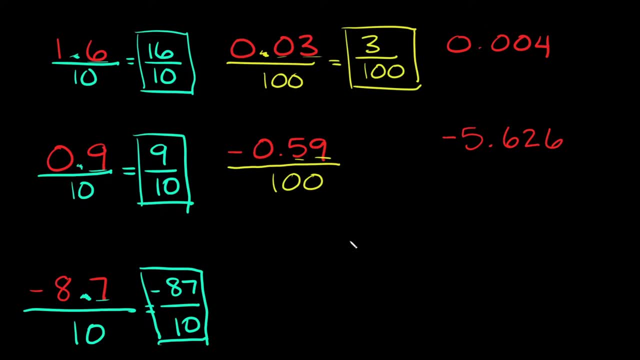 ends right. so it ends in the hundredths. so that's what goes in my denominator, and then my answer would be again, just drop the decimal. negative zero, five nine. but I'm just gonna drop the zero because it doesn't add anything. so it's just actually gonna be negative: 59 over 100. 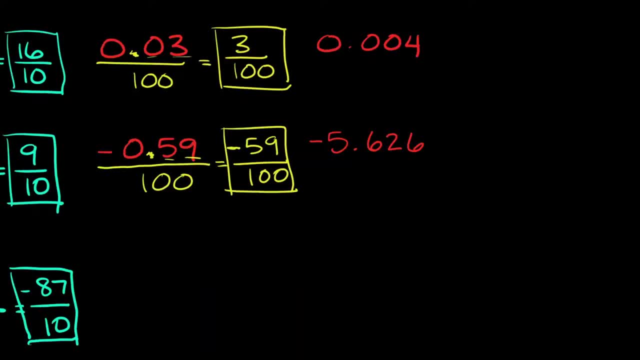 okay, so this would be your answer. okay, now we just have a few more examples, so I'm just gonna move over to the side a little bit here. okay, so now up here on the right we have 0.004. so again, I'm just gonna draw a line underneath my 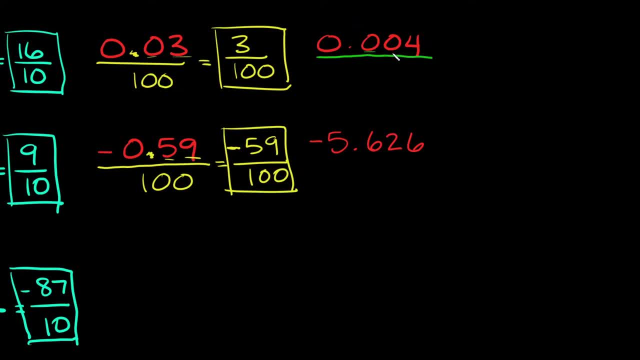 whole number and what place value does this end in? well, let's see tenths, hundreds, thousands. so this ends in the thousands place. so I'll put a thousand on the bottom, all right, and then just rewriting my answer. remember, drop any of these leading zeros and this decimal point right there. so we're just gonna. 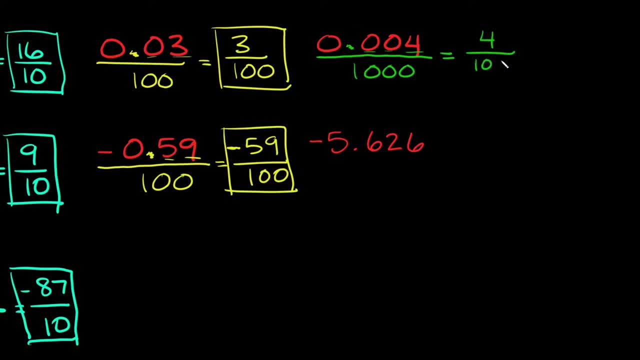 have four on top and a thousand on the bottom. so your answer here would be four over one thousand, okay. and lastly, here we have negative five point seven, six, two, six. so draw a line underneath the whole thing. it ends in the thousands place. so we'll put a thousand in the denominator and then this is: 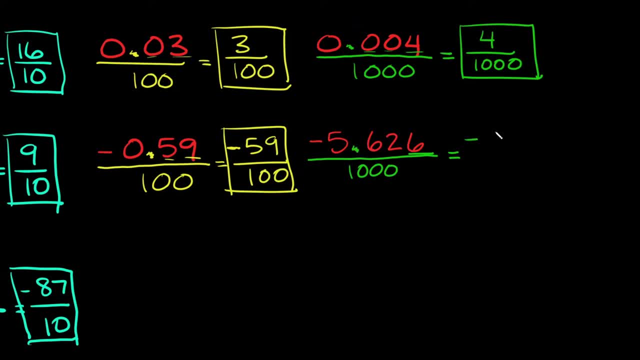 gonna be equal to dropping the decimal negative five six, two six over one thousand. okay, so, negative five thousand six hundred twenty six over one thousand. that's your answer, right there. all right, guys. so that's a quick and easy way to convert decimals to proper and improper. 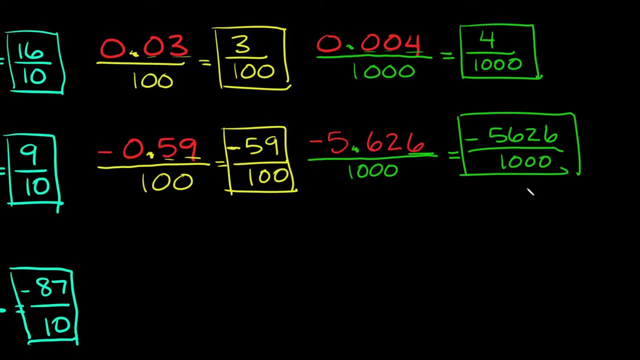 fractions right. so I hope the video was helpful. if it was definitely, leave a thumbs up down below, and if you still have any other questions, leave them in the comment section below and I'll do my best to try and help you out. there's also a playlist attached at the end of the video, so if there's any other topics, 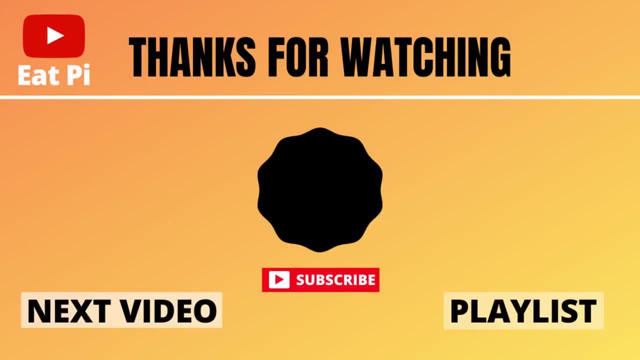 you need help with. definitely check those out and I'll see you there. you.